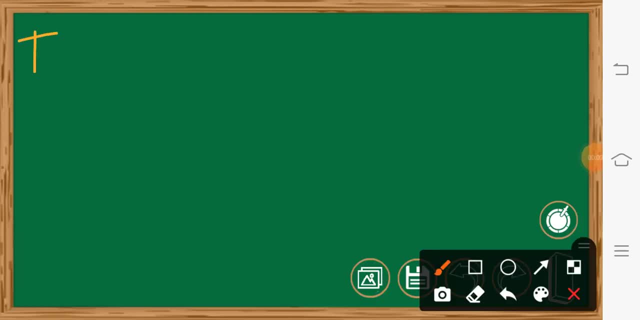 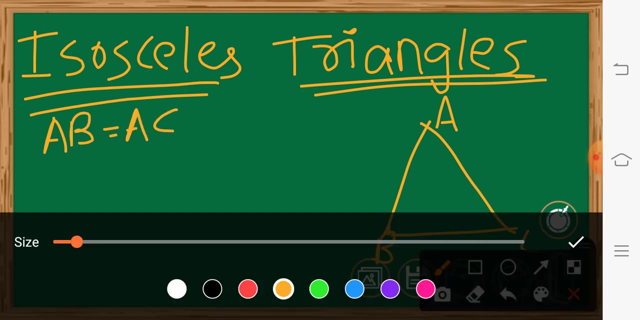 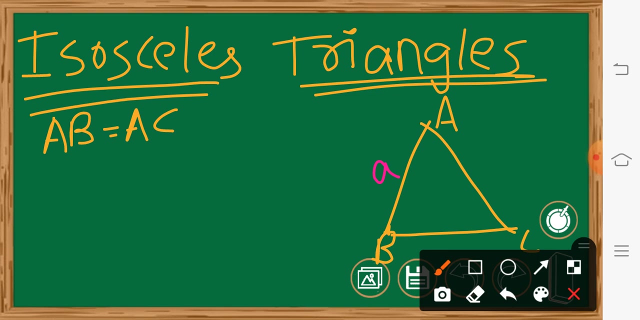 Isosceles triangle. Isosceles triangle is a triangle which has two equal sides. That is called isosceles triangle. Here, this ABC triangle is a isosceles triangle. AB length is equals to AC length. We assume AB length is equals to A, Then AC length also equals to A because these two sides are equal. But this is different. So it is B. This length is equals to A. Here this is height of this triangle: H. 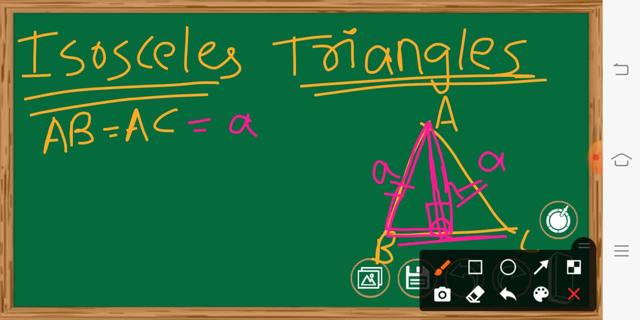 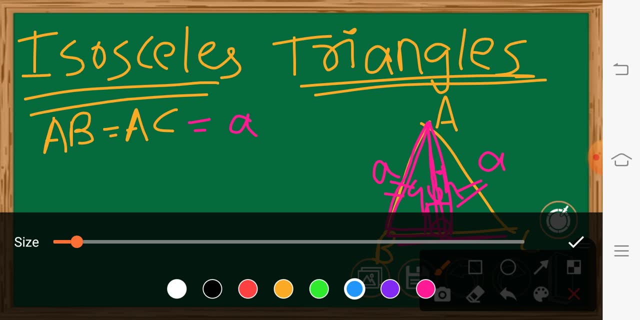 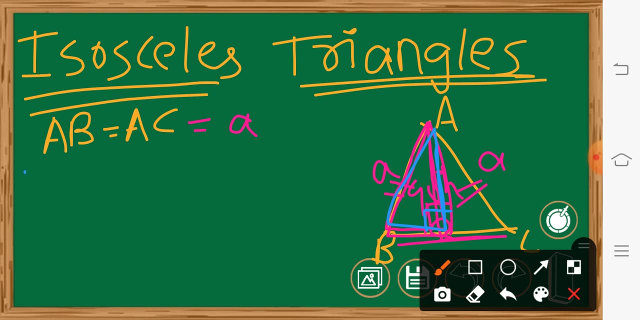 We get this right angle triangle here. this is 90 degrees by the Pythagoras theorem. this is right angle triangle. by the Pythagoras theorem we get height value. height of this isosceles triangle is equals to half into and the root of 4 a. 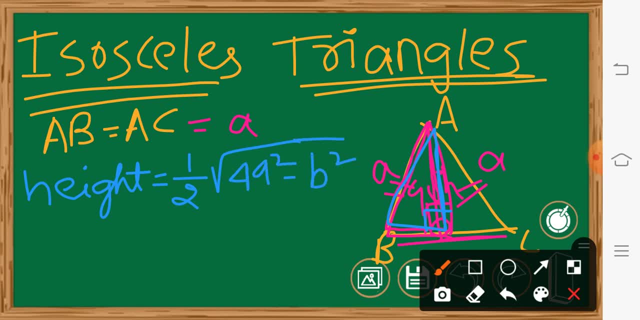 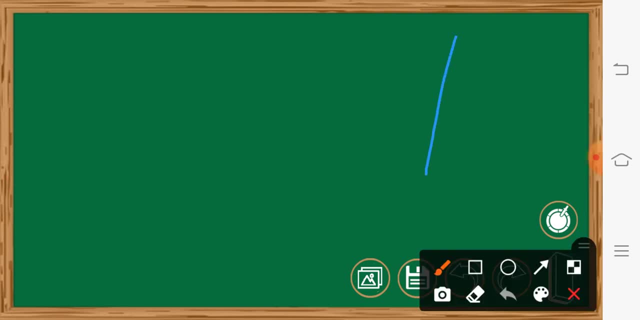 square minus b square. this is formula for height. next, area of isosceles triangle. this is a isosceles triangle. in this triangle, this two lengths are equal. so area: this value is A. this is equals to A. this is B. formula for area of triangle is equals. 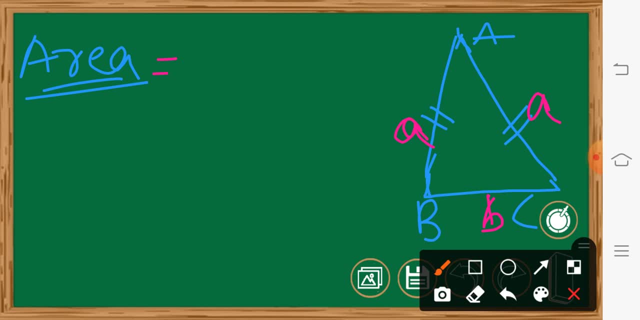 to half, into base, into height. by that formula we get: area is equals to b by 4 and the root of 4, a square minus b square b. what is the base value here? b, this is b, this is a. if a is equals to four centimeters, that means this side length, ac side length, is equals to four centimeters. 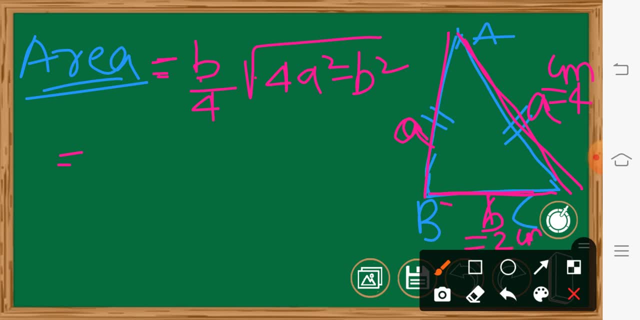 b base value is equals to two centimeters. this length is two centimeters, then what is the area of this triangle b? b equals to base, so two by four on the root of four into a value. also, four, four square. minus b is equals to two is equals to two square, if we cancel. 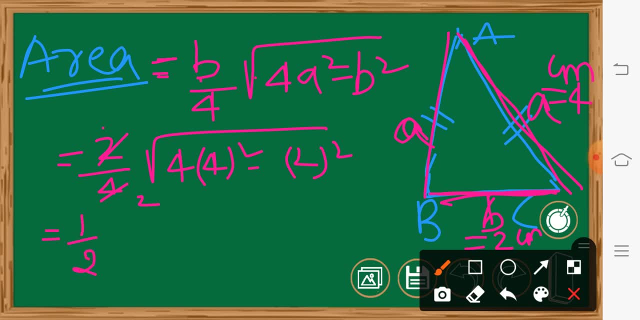 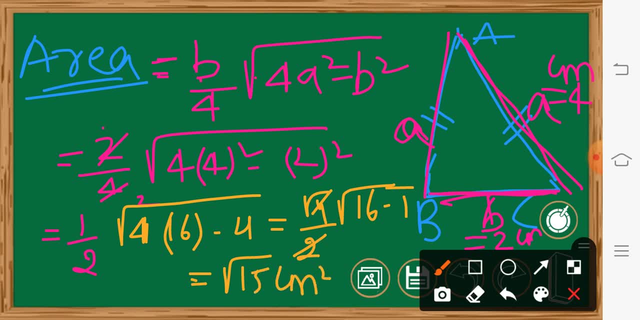 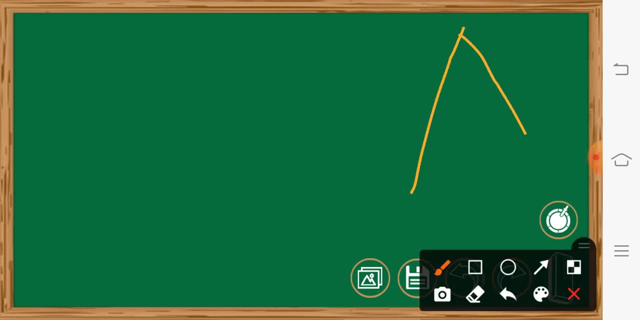 to root 그냥 square. square is the area of this triangle, now perimeter. perimeter, perimeter of this isosceles triangle is sum of all sides. that means this side, this side and b c side, three sides. perimeter is equals to sum of all sides: a, b plus b c plus. 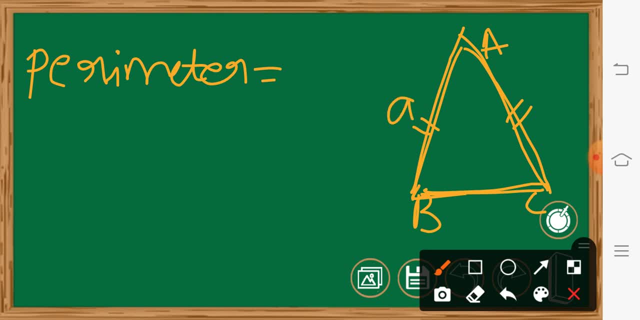 a, c. so a b value is equals to a, a c value equals to also a b. c value is equals to b. a plus b plus b, that equals to two a plus b. if a value is equals four centimeters, b value is equal to two centimeters. then what is the perimeter of this triangle? two into. 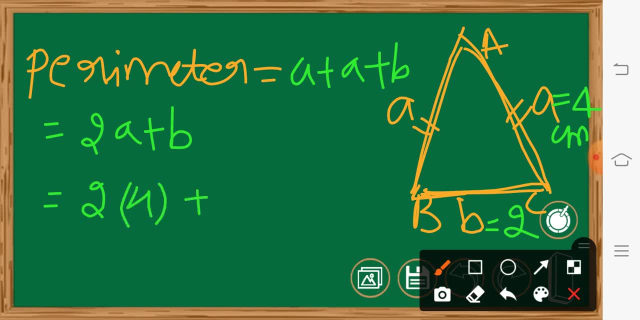 a value is equals to four centimeters plus b value is equals to two centimeters. so two fours are eight. plus two, that equals to ten centimeters. this is the perimeter of this isosceles triangle.